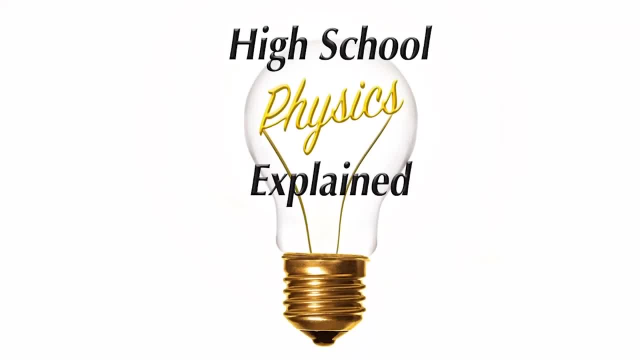 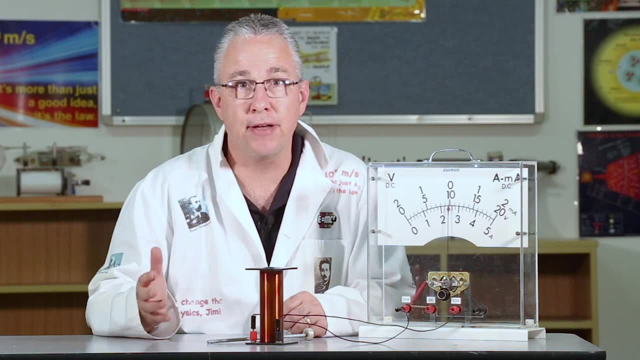 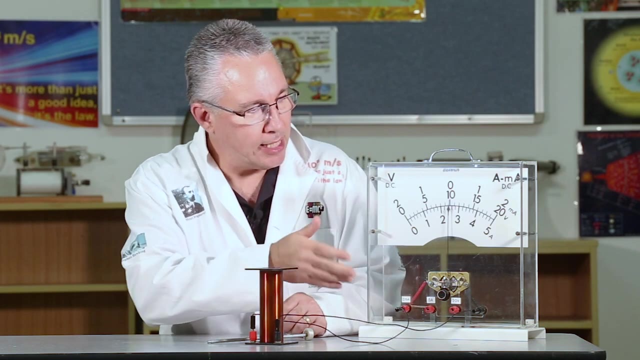 Hi and welcome to High School Physics Explained, and today I want to demonstrate Faraday's Law and give you a bit of an explanation as well. So in front of me I have a coil and that is connected to this ammeter or galvanometer. 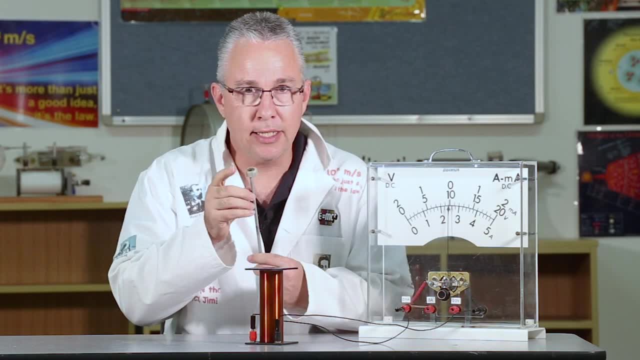 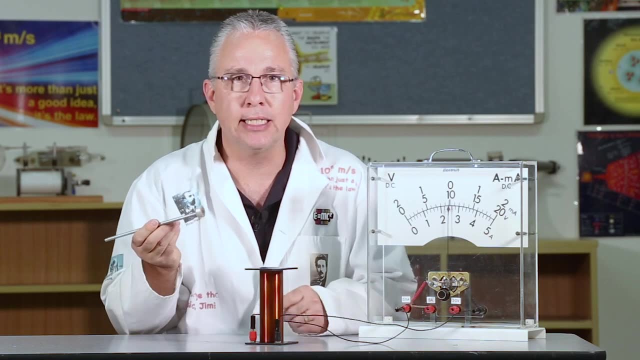 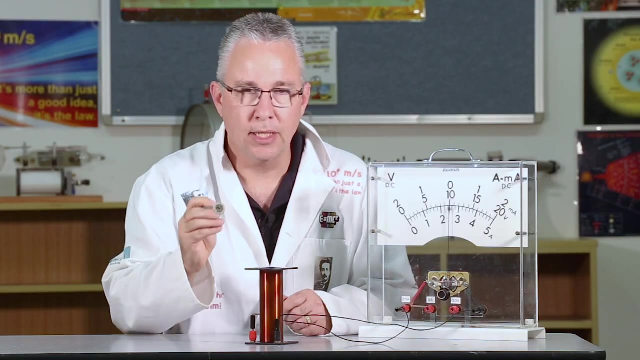 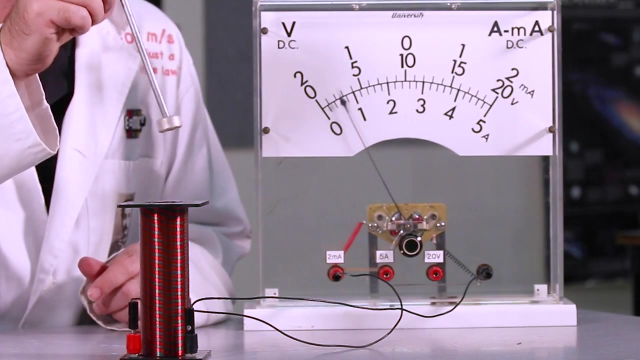 And I also have a rare earth magnet and this magnet is facing so that the north is facing outward, like. so What's going to happen when I insert this magnet into this coil? You see the needle deflect. What if I do this faster? You should see that the needle deflects a greater amount. 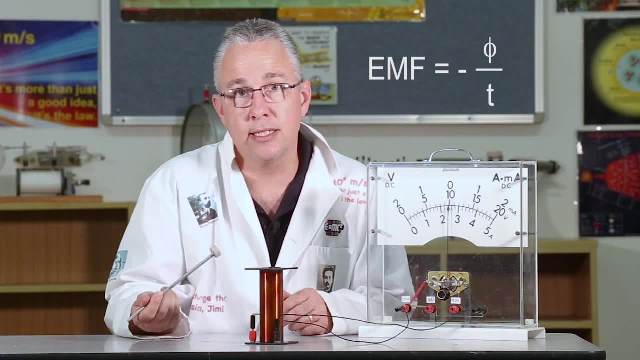 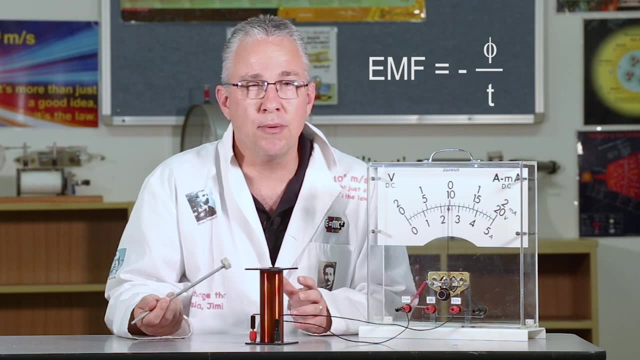 So what's going on? Well, Faraday's Law in essence says that the rate of change of flux causes the production of an EMF, or in other words, what is commonly referred to as an electromotive force, though in reality it's talking about a voltage. 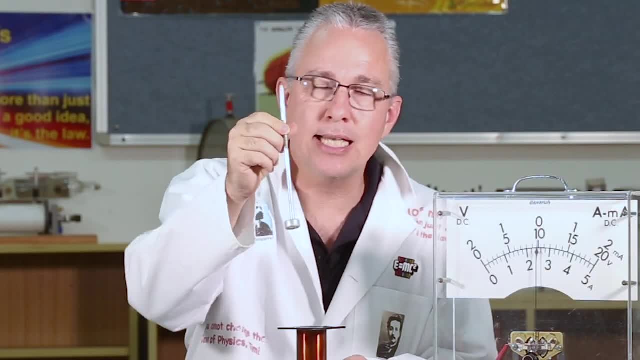 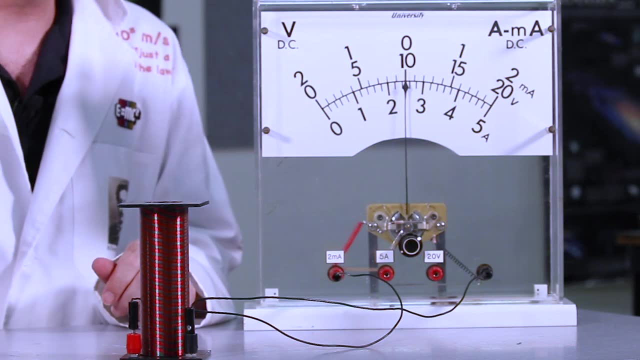 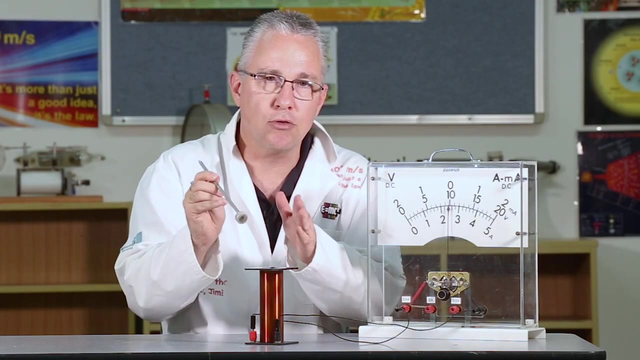 So when I place the magnet in the magnet has a magnetic field around it. Magnetic field lines are radiating around out from the magnet And as I insert the magnet into the coil, the coil experiences a change of flux. That is, these magnetic field lines are crossing over the wires. 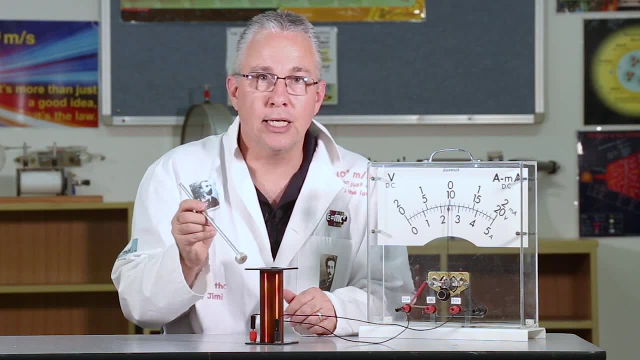 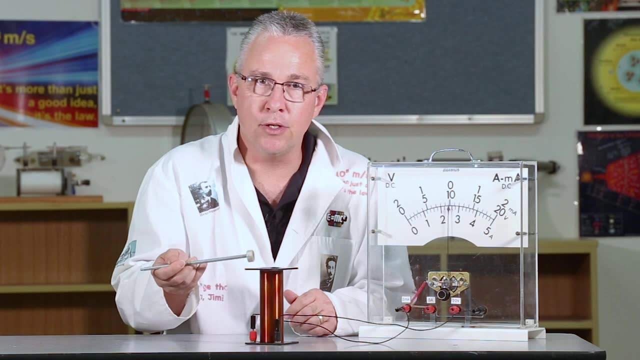 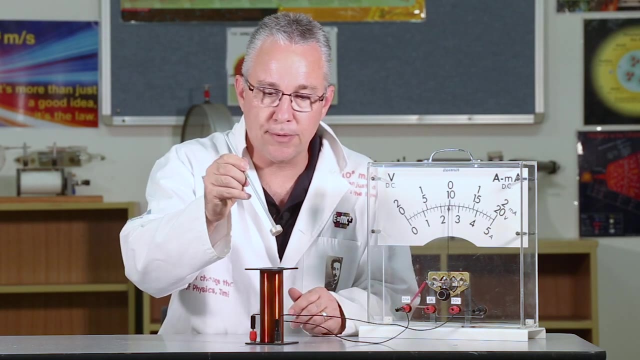 And the rate at which that occurs is causing a production of an EMF. Now, EMF is like a voltage, So since I am producing a voltage and we now have a closed circuit, I'm also producing a current as a result, And so we see that in the deflection. 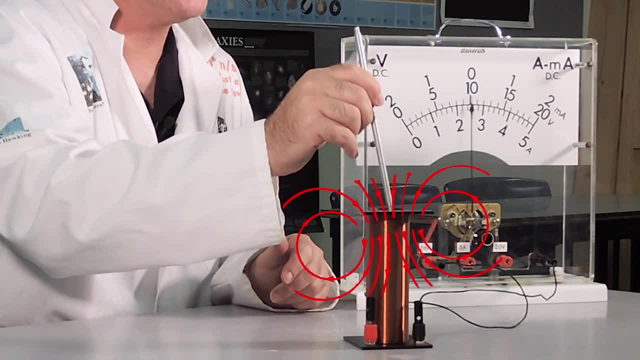 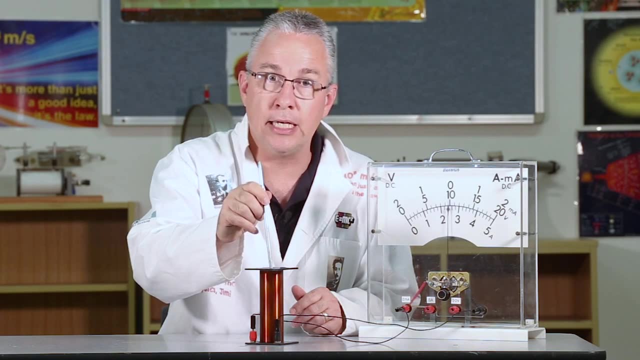 Now, the direction of the magnet or the direction of the relative motion between the magnetic field lines and the wires determines the direction of the EMF and hence the current. So if I pull it out, you're going to see it deflect the other way. 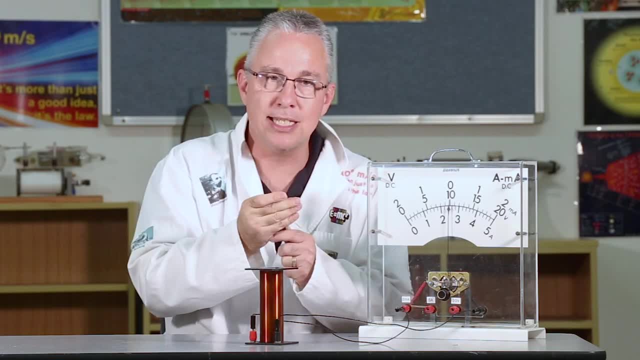 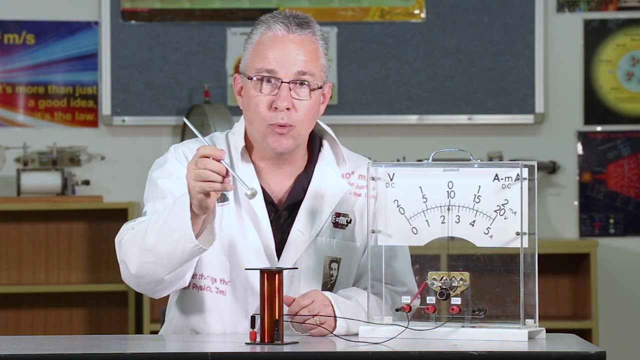 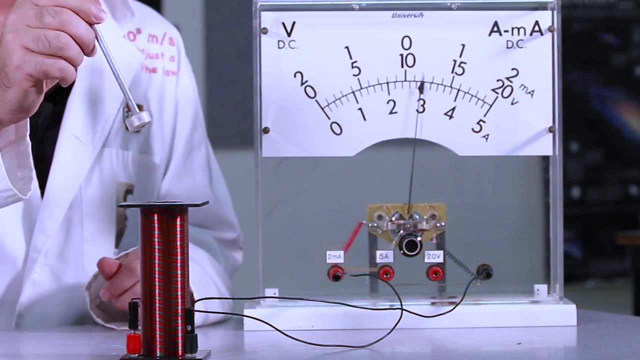 Now what will happen if I turn my magnet over, so that the south is now facing outward? We're going to see the same effect, with one small exception, That is, the deflection will be in the opposite direction. Why? Again, because the magnetic field lines are now in the opposite direction. 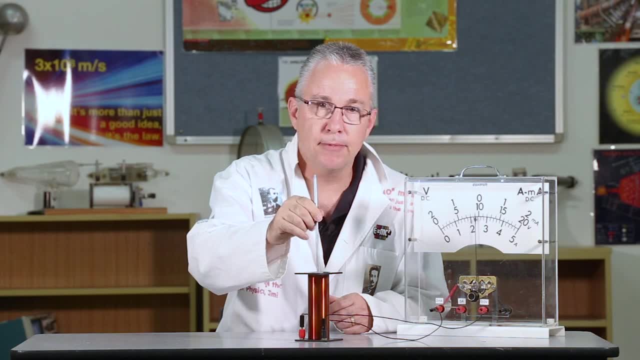 Now what happens if I hold it stationary? You'll see no deflection whatsoever. That's because we don't have any changing flux. We don't have any rapidly changing magnetic field lines crossing my wire, And so I have no EMF. So that's a very simple demonstration of Faraday's Law. 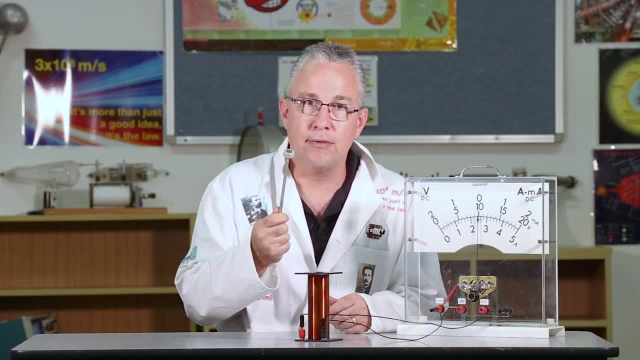 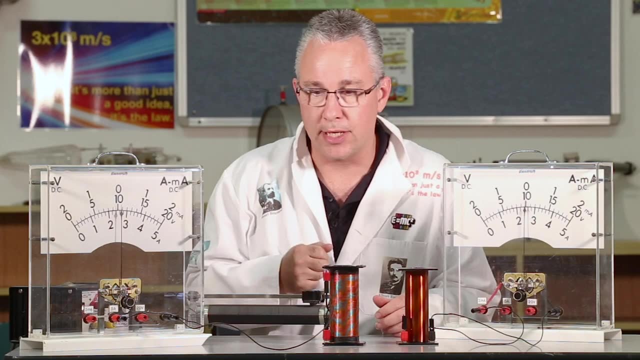 But let's say I don't want to use a magnet to generate a rapidly changing flux. What can I do then? And now, in a variation of Faraday's Law demonstration, you'll see I still have my solenoid over on this side, connected to the ammeter. 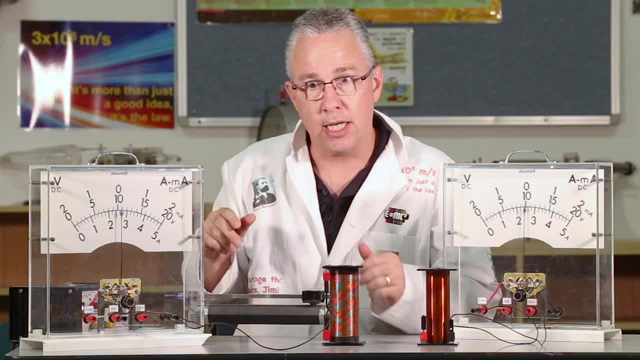 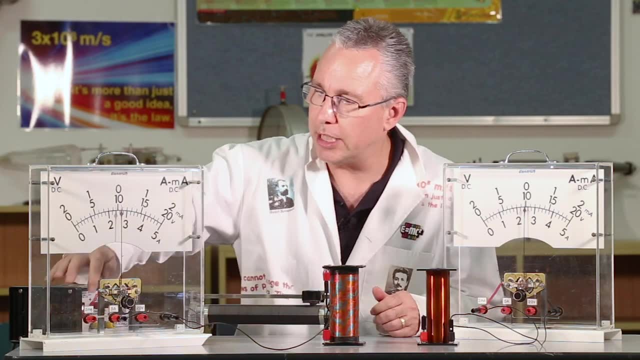 and there's no connection to a power supply. On this side, I have an ammeter, a solenoid and a rheostat which allows me to control the amount of current. So if I turn it on, I'm going to get a deflection, as you would expect. 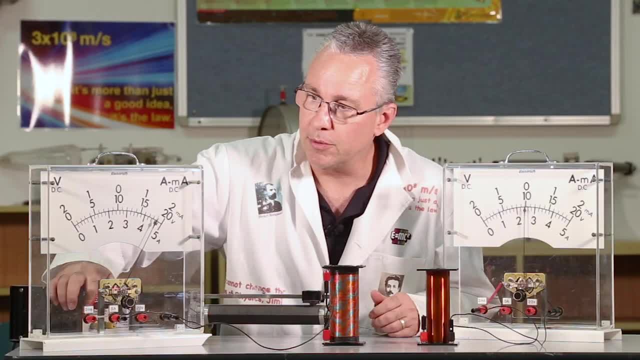 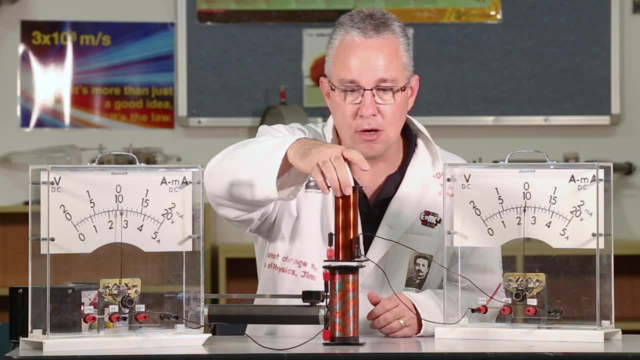 A current is flowing through the solenoid And of course it will turn to zero when I turn it off. Now what happens if I place this on top of the solenoid, like so? There's no connection to the bottom solenoid. 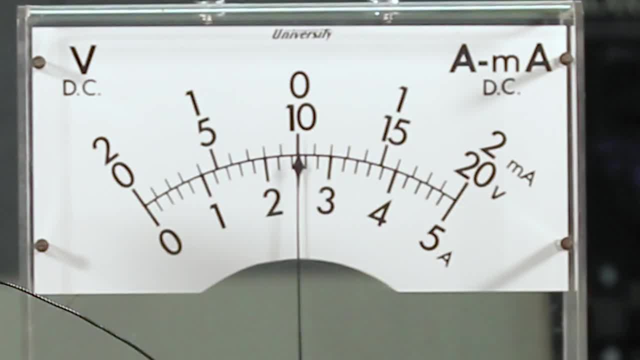 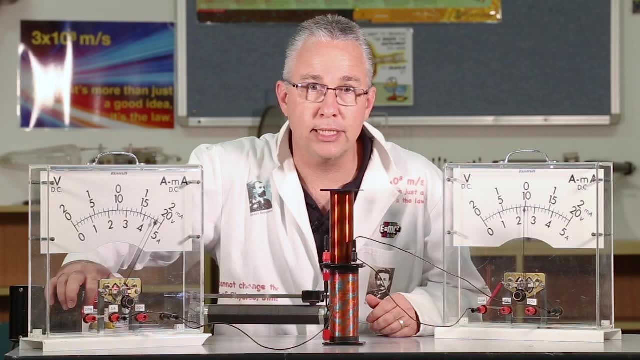 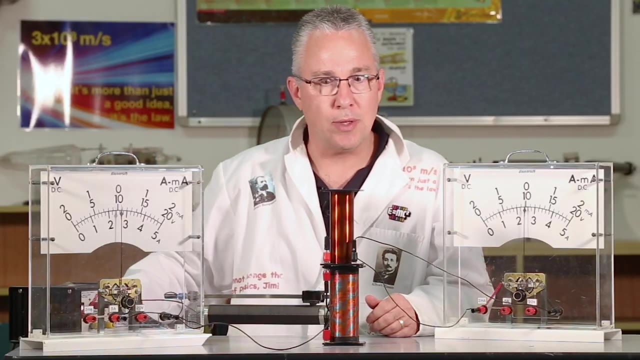 Let's see now what happens. when I switch it on. You may have noticed that a very, very slight deflection takes place, But the deflection lasts only momentarily. Now I'm going to accentuate the deflection Now. this is just some metal rods. 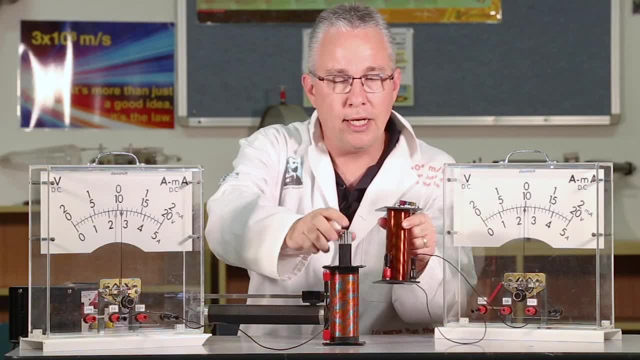 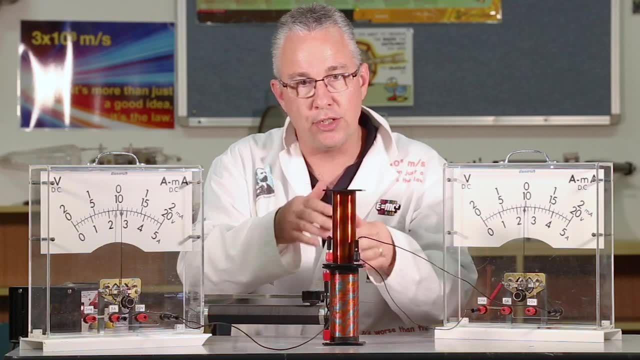 And I'm going to place them in the centre of the core. Now, these are not causing these two solenoids to be connected electrically. In other words, there is still a separation of two different circuits. The only thing I've done is inserted some metal core. 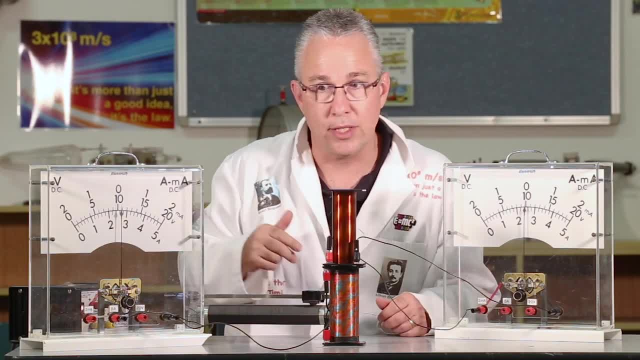 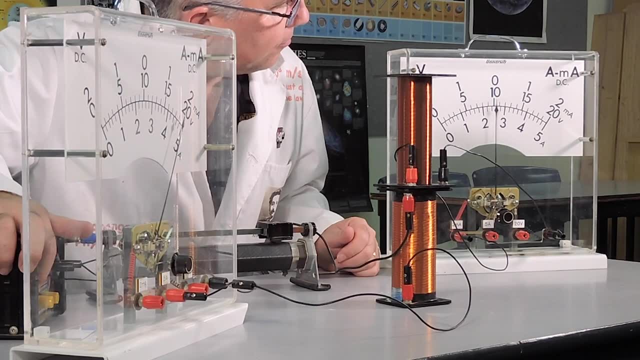 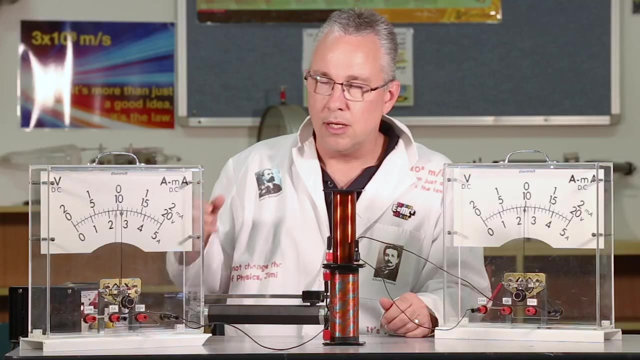 which is going to concentrate my magnetic field lines, And I'm going to demonstrate this when I turn it on Again. watch what happens to the meter over here. Now, when I switch it off, what do you notice? Well, the first thing is that the direction of the deflection 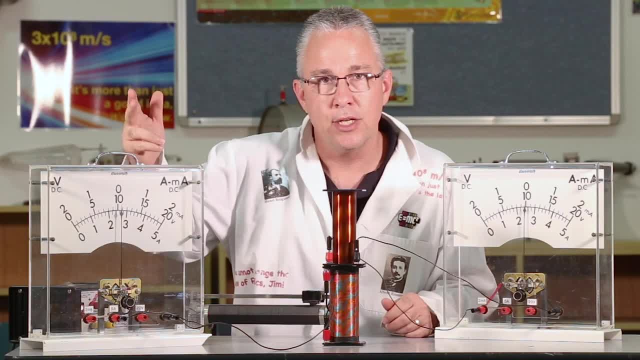 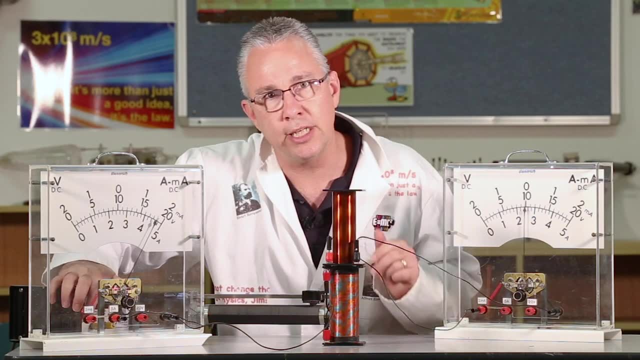 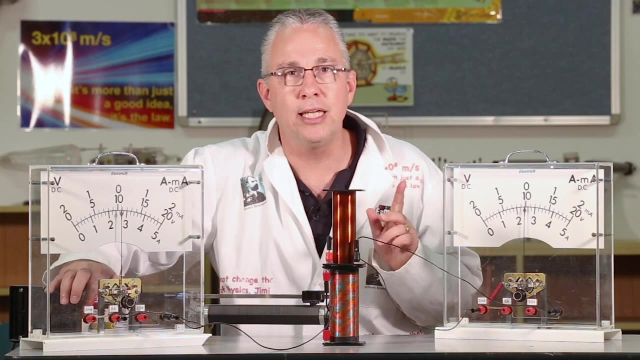 is opposite to the direction of the current. So the current that is going to go from this circuit is clearly going in the positive direction, But the deflection here occurs in the negative direction. When I switch that off, you're going to see that the deflection heads in the positive direction. 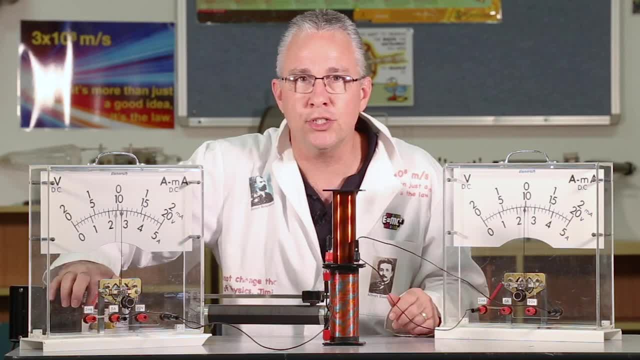 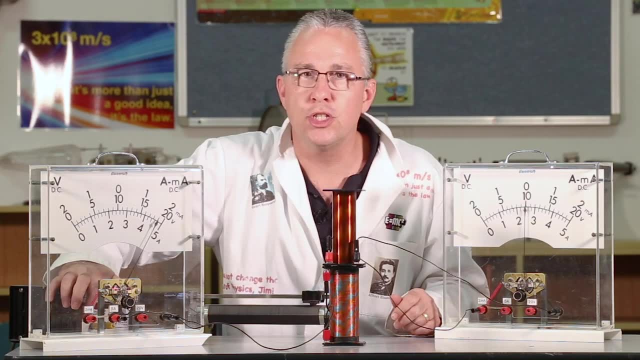 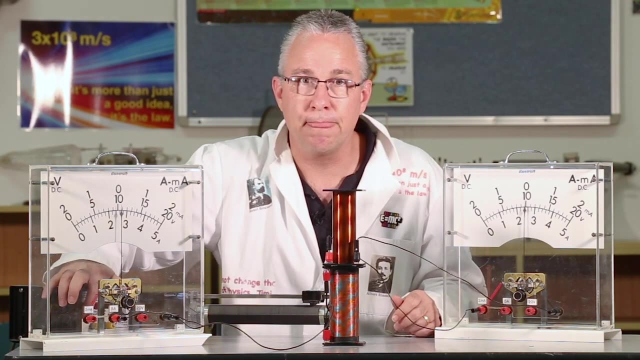 The other thing you might notice is that the deflection only lasts momentarily. It lasts for about the time that I'm switching it on, but returns quickly to zero. Similarly, when I turn it off, it deflects and returns back to zero. 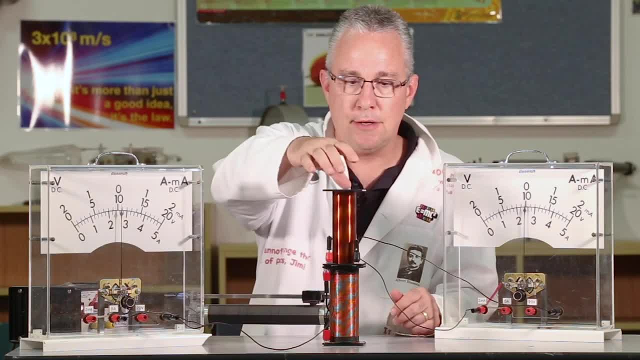 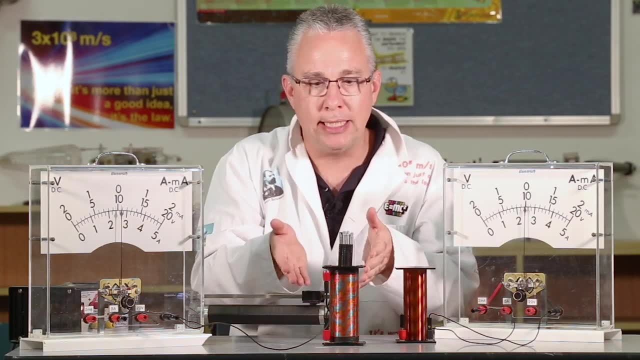 Again, let's explain what's going on. If I just pull this out of the road, when I turn this on, we start with a situation where we have no magnetic field lines. But when I turn the current on, we are having a developing magnetic field. 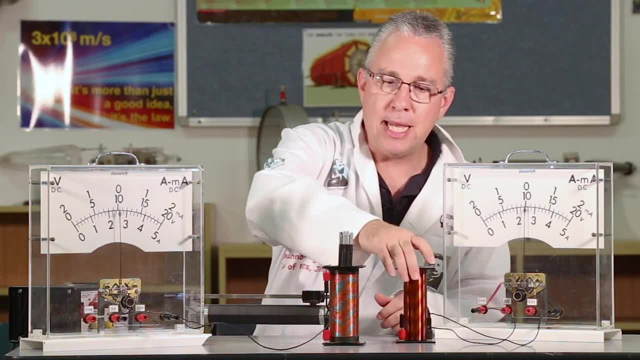 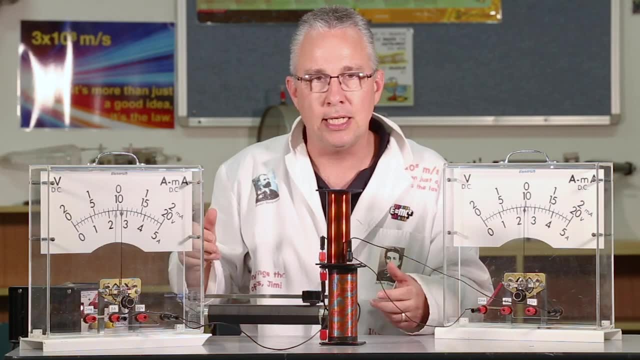 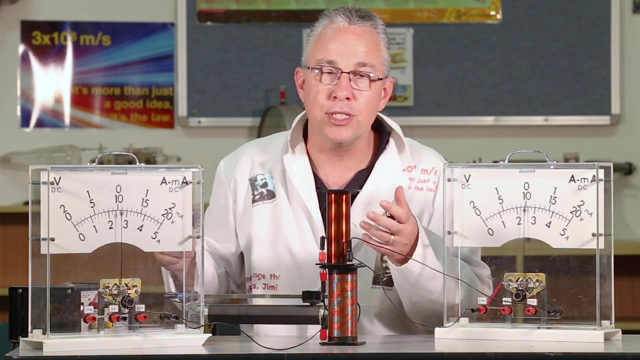 a growing magnetic field. If I place my coil in the midst of the growing magnetic field that this bottom solenoid is generating, this top coil is experiencing a rapidly changing flux, and the rate of which, of course, is determining the EMF that is generated. 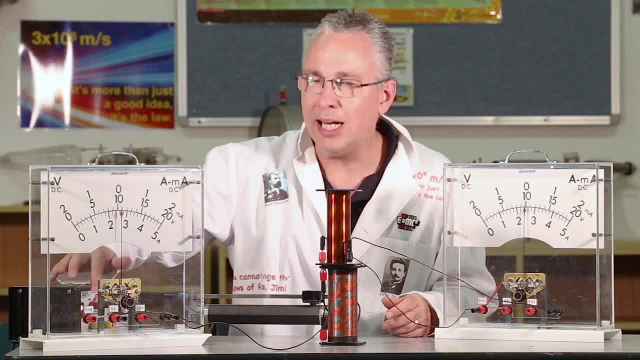 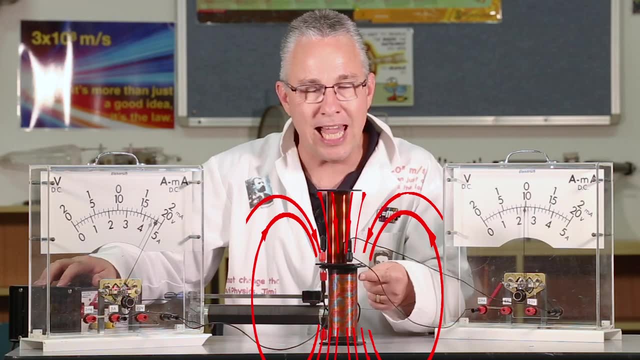 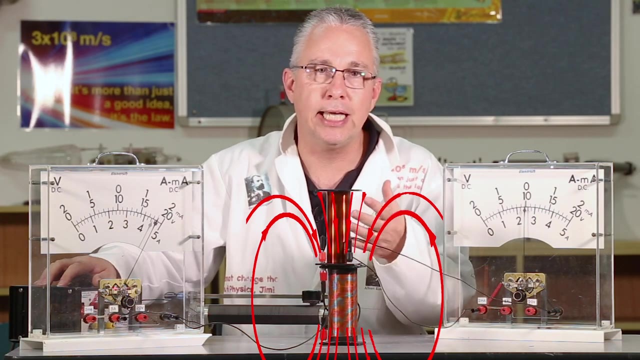 and, following on from that, the current that we get. But when I leave, the power on the current is steady, which means my magnetic field, which is still there, is not changing. it's staying steady, which means the top coil is not experiencing any changing flux. 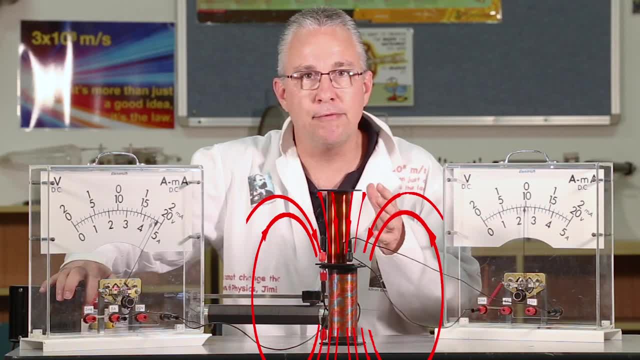 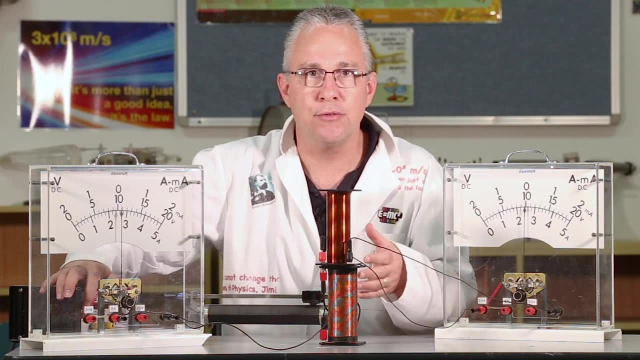 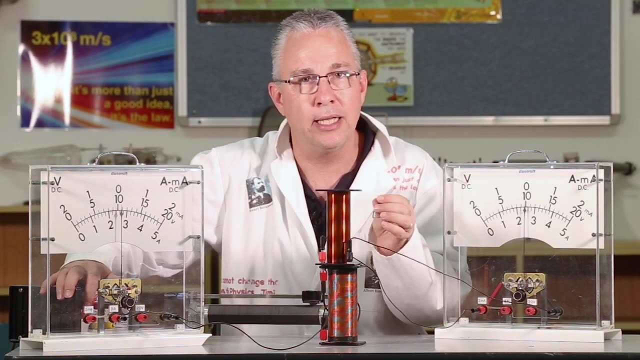 What if I turn it off? Well, I suddenly go from a very large magnetic field that this top coil is in, that is going to rapidly decrease to a point of zero, because the current, of course, switches off Again. it's not an instantaneously disappearing magnetic field. 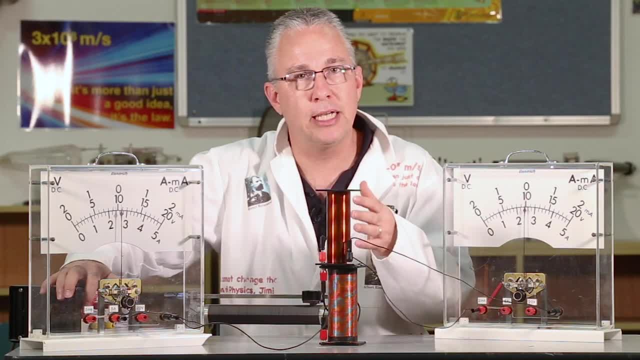 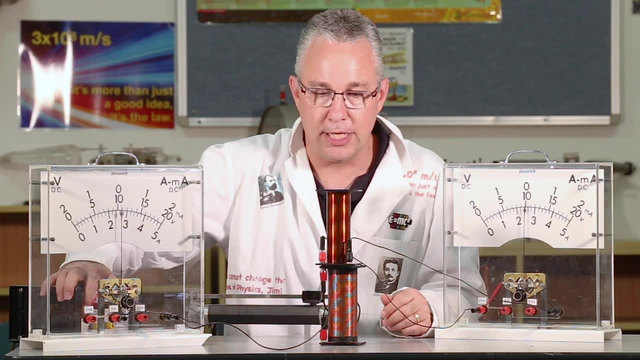 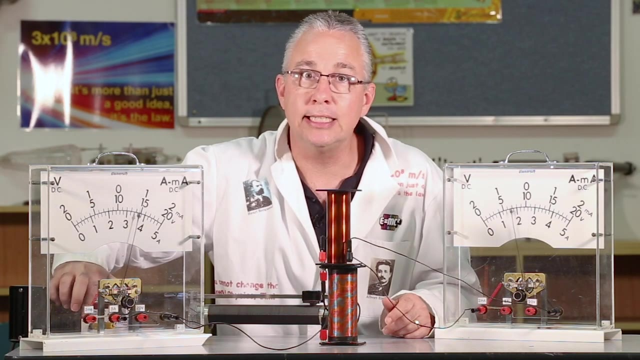 It drops away, which means the top coil is now experiencing a rapidly changing flux in the opposite direction. Hence the needle will deflect in the opposite direction. So turning on and off rapidly will give me an alternating current. I have a video on the induction coil. 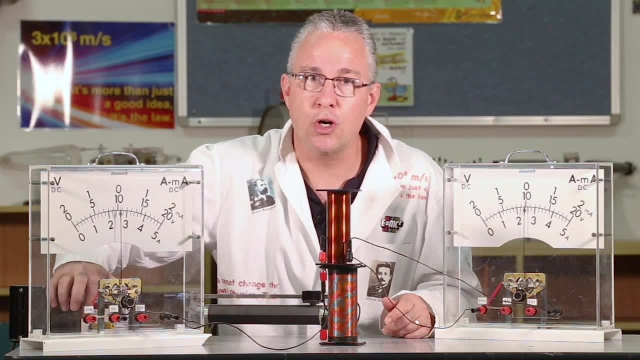 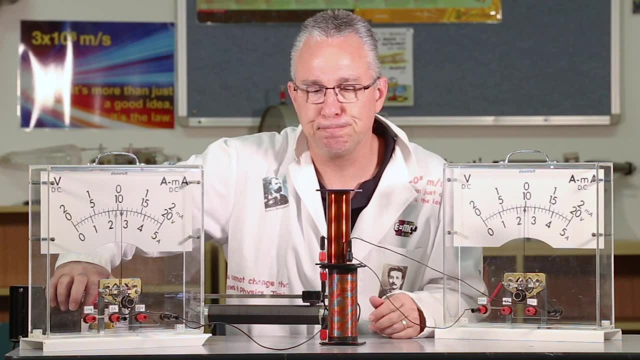 which in essence, works on the same principle. Switching it on and off on rapidly will cause me to have an induction, that is, an alternating supply in the top coil. The last thing I want to mention is the concept of Lenz's Law. 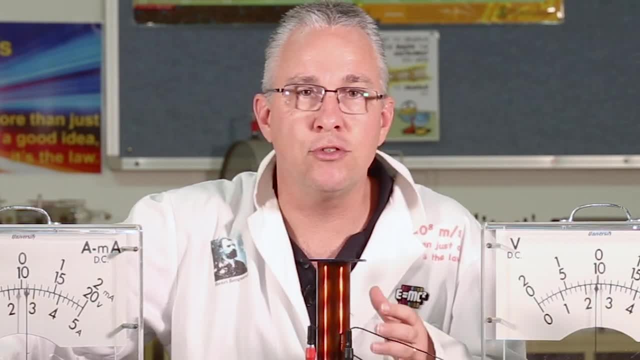 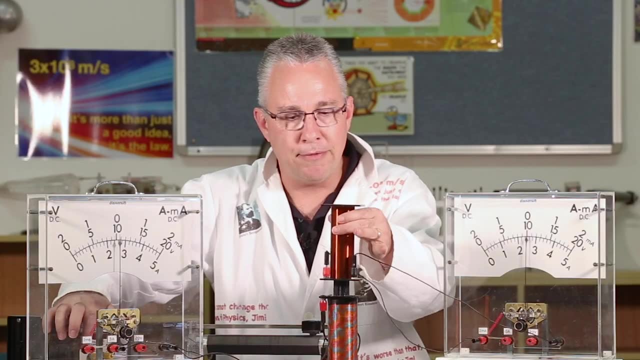 And Lenz's Law is such that whatever generates the magnetic field, an EMF is generated so that it opposes the change. So if I were to lift this up like so and I were to turn this on, this would generate a magnetic field. 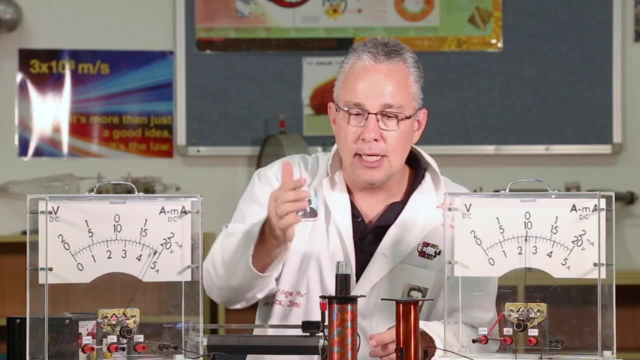 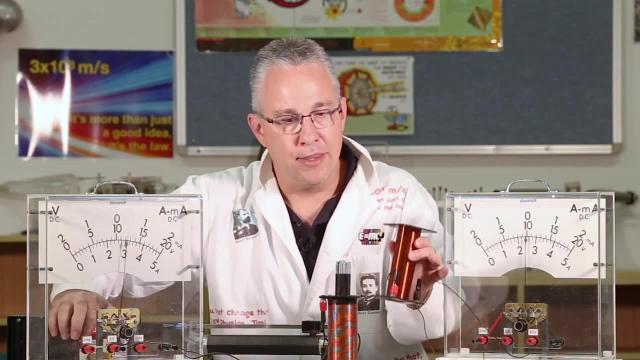 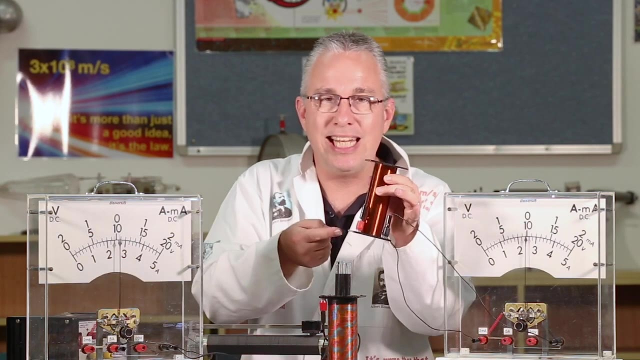 if the current was going in the direction of that. I'm going to get a current that causes the top section here to be a north pole. This one will generate an EMF, But the result is is that the current that's generated will produce a pole in the opposite side. 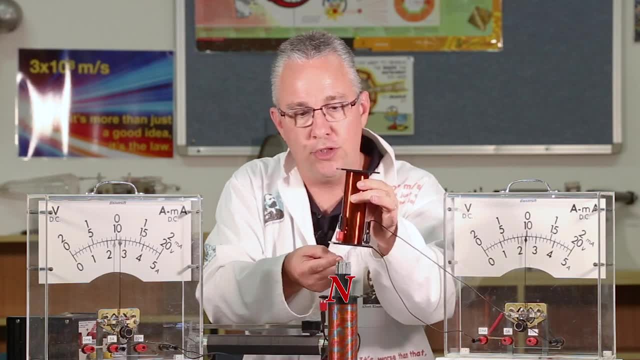 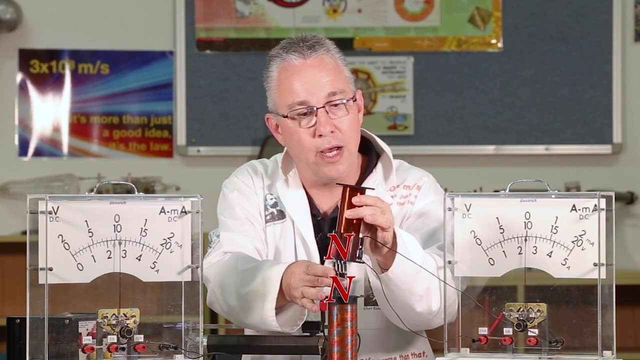 It negates it. So, in other words, we're going to get a north pole generated at this point as a result of the north pole being generated at this point, which is the reason why the current is going in this direction. It's going in the opposite direction. 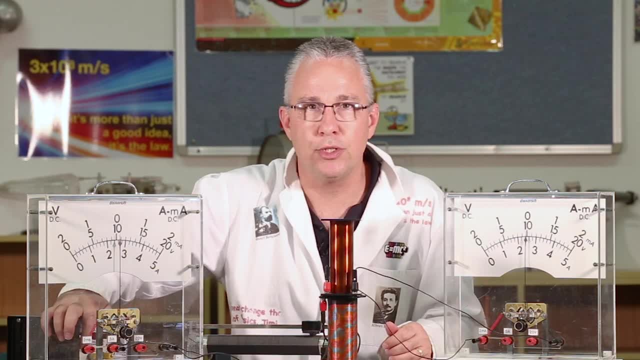 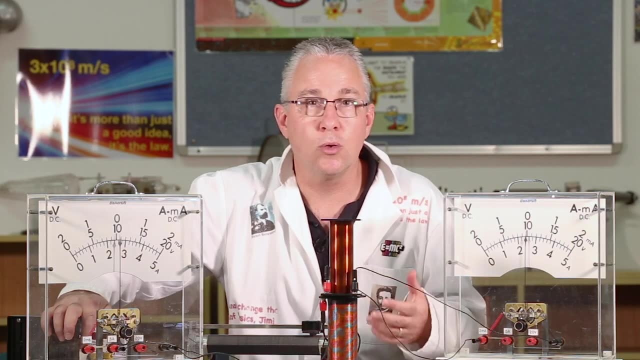 when I switch it on, Similarly speaking, if I switch it off, That's a very important principle, Lenz's Law, because it actually is a follow-on from the Law of Conservation of Energy. Now I have a video that discusses Lenz's Law. 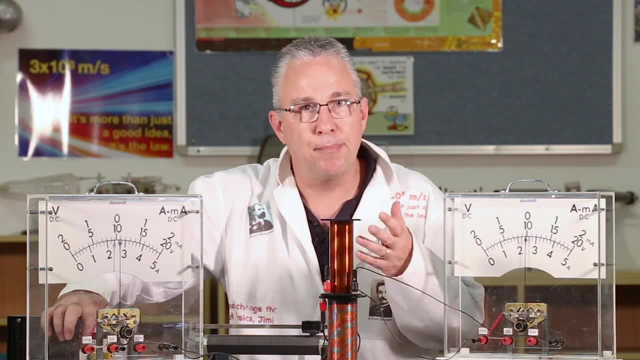 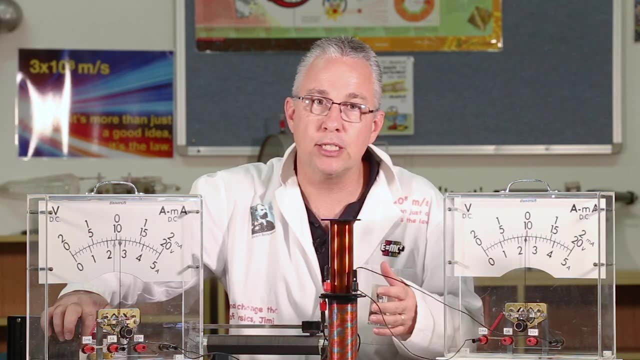 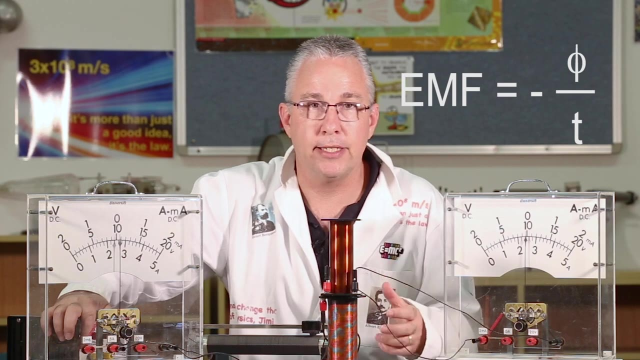 in greater detail and I encourage you to watch that. But both demonstrations that I've now shown you is a demonstration of Faraday's Law, That is, the rapid change of flux with respect to time will cause an EMF And the negative sign in the formula of Faraday's Law. 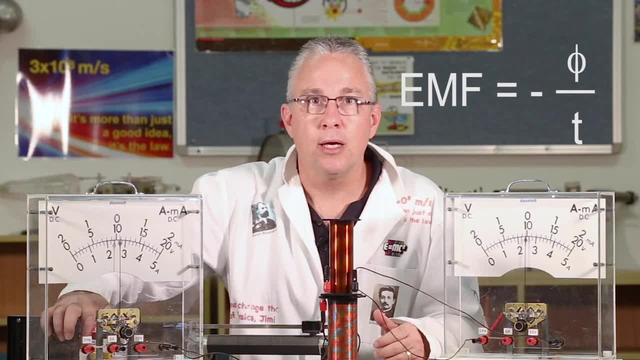 signifies Lenz's Law. Well, I hope that has helped you understand a little bit more in detail of Faraday's Law. I'm Paul from High School, Physics Explained. Please like, share and subscribe. Have a look at some of my other videos. 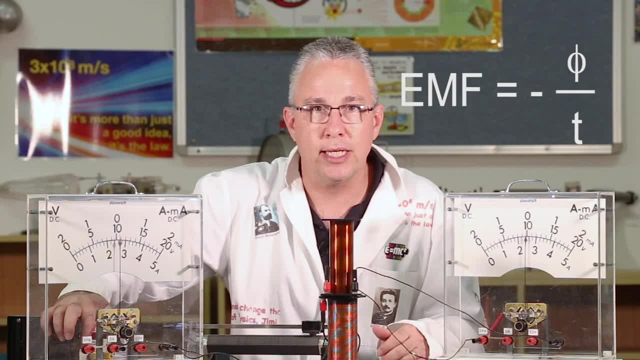 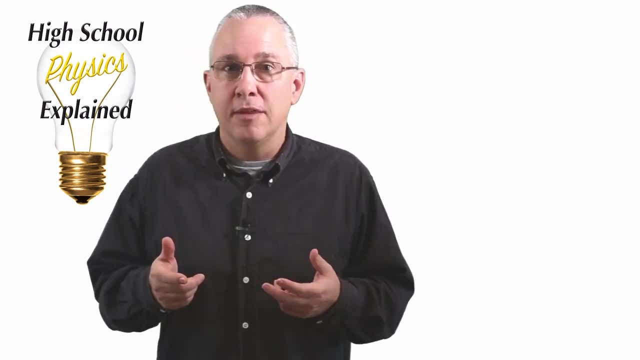 Specifically, I have a number of videos to deal with electromagnetism. Any case, thanks for watching. Bye for now. Well, I hope that helps you understand the concepts. Thanks for watching. Please remember like, share and subscribe And, by the way, drop a comment down below. 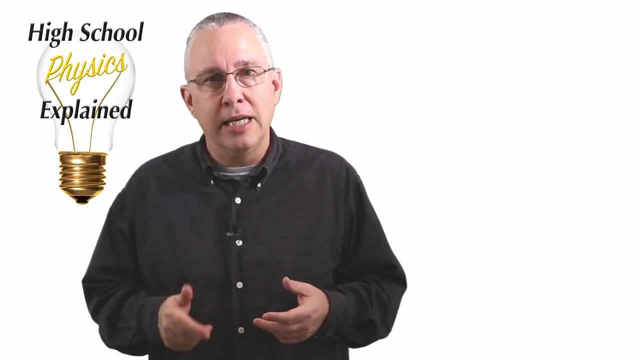 if the video particularly has been useful, And finally, consider supporting me via Patreon. The idea is to develop resources and equipment to continue to teach physics at a high school level. I'm Paul from High School Physics Explained. Bye for now.